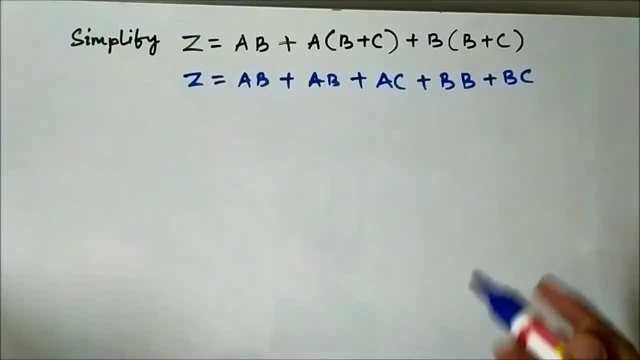 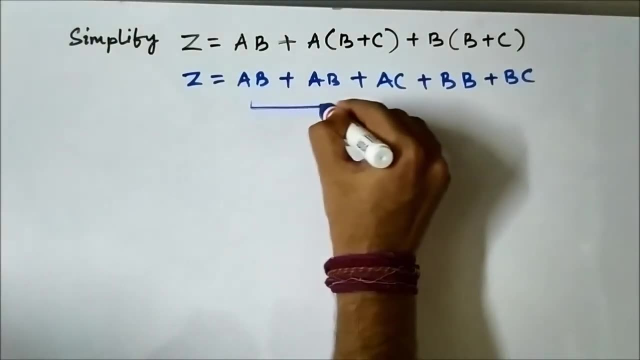 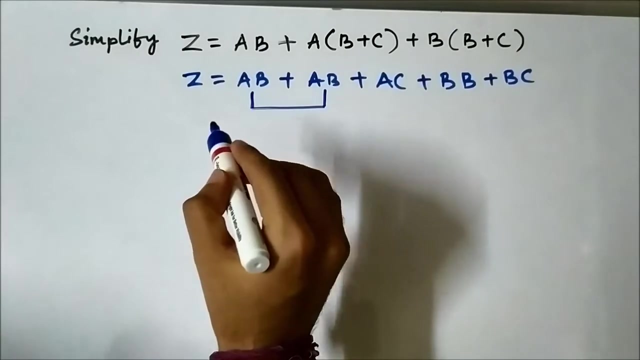 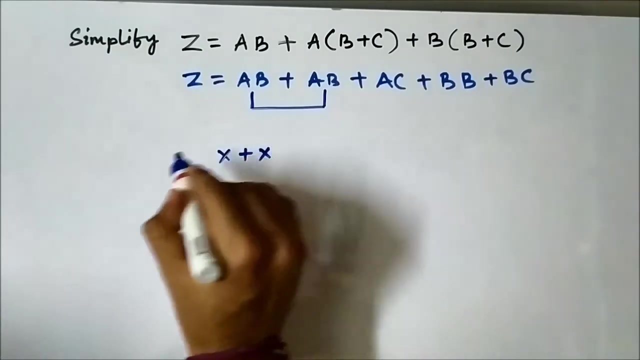 and operation. Okay, Because it is the digital electronics Boolean algebra. Okay, So focus here. here a Boolean algebra rules will come into play. we know that the or rule according to one of the or rules if 2 Boolean variables in same one with the same Boolean variables. 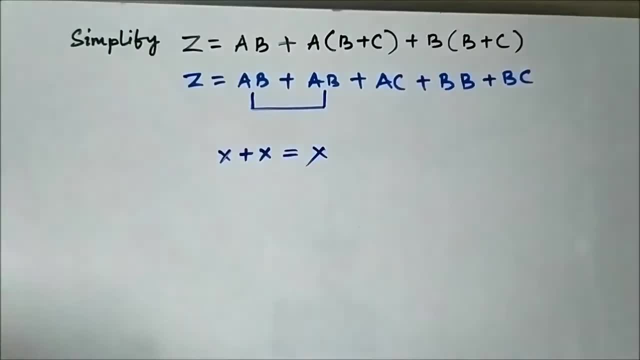 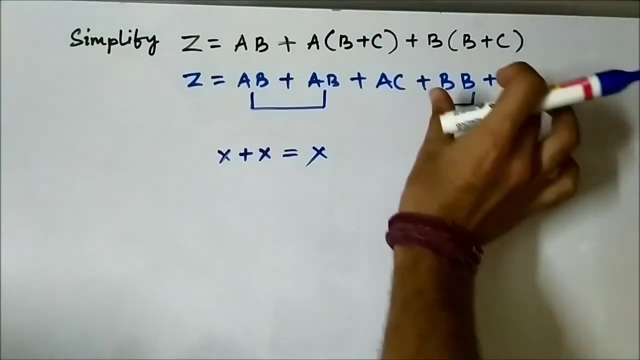 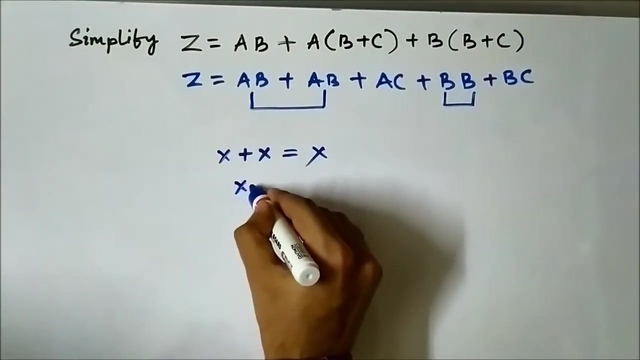 they get, or together it will result in the same Boolean variable. x plus x is equal to x. So here 2 ar, bar, h, t, z, 6 on x plus x, 0.ee boolean. same boolean variables are anded together. okay, it means it will result in the same boolean. 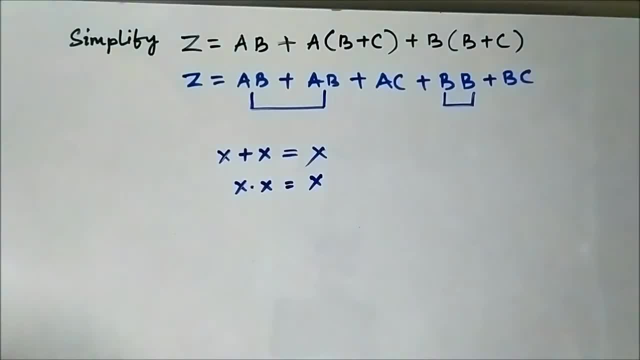 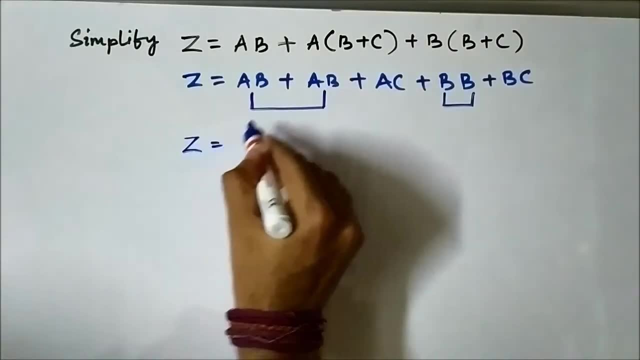 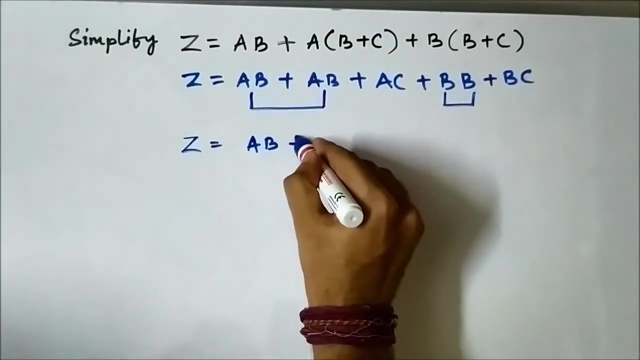 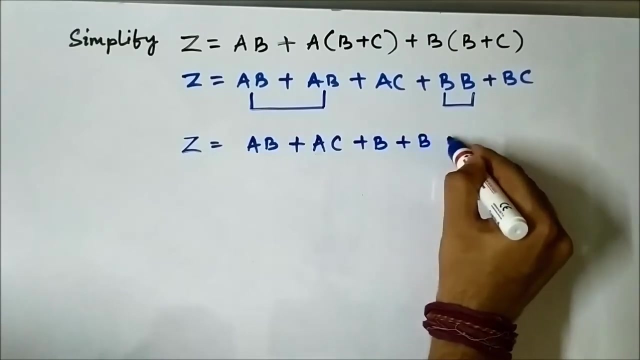 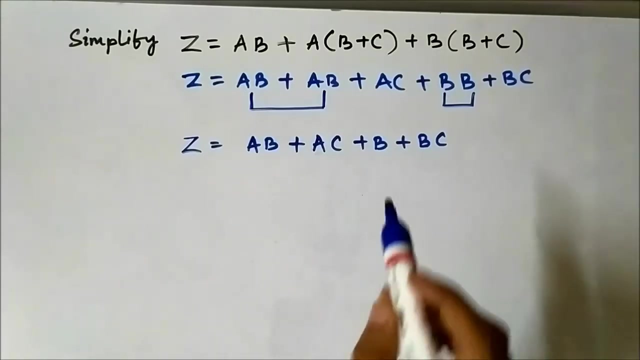 variable. okay, so here we can apply the boolean rules. so how it will come up? it will be equals to ab. okay, these two added up result in ab plus ac plus b plus bc. okay, now, here we will apply this focus. here we will apply the absorption rule. now, what is the? 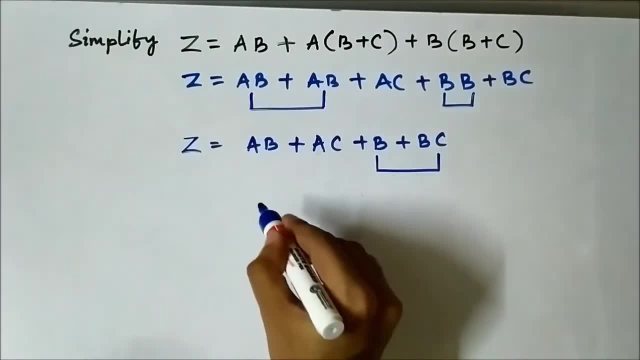 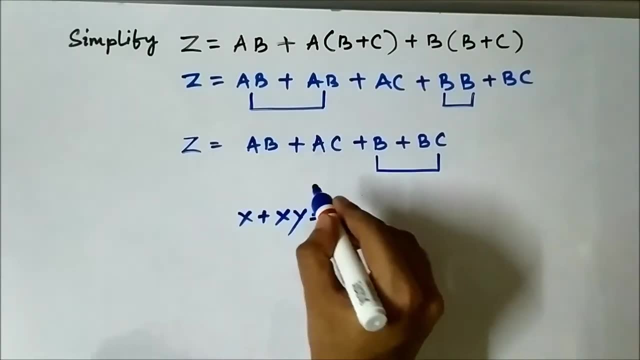 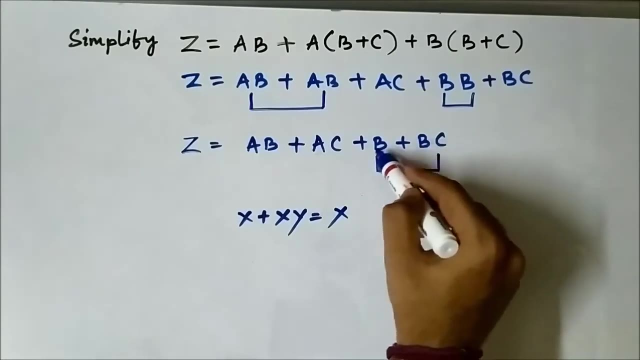 absorption rule rule. it says this: let us say x and y are two Boolean variables, then this will be equal to x. here identify the pattern here: b plus b, c. here it will be b, x plus x, y equals to x. so I have already discussed these rules, so you please watch those videos where I have discussed. 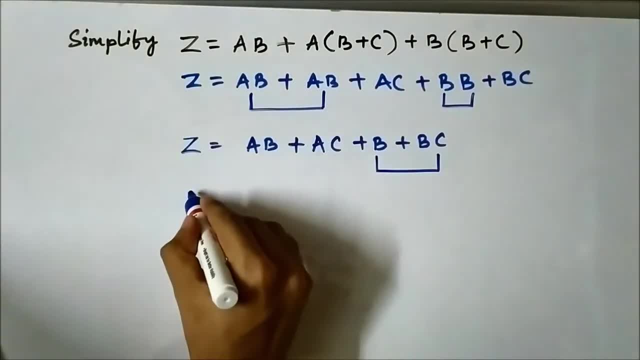 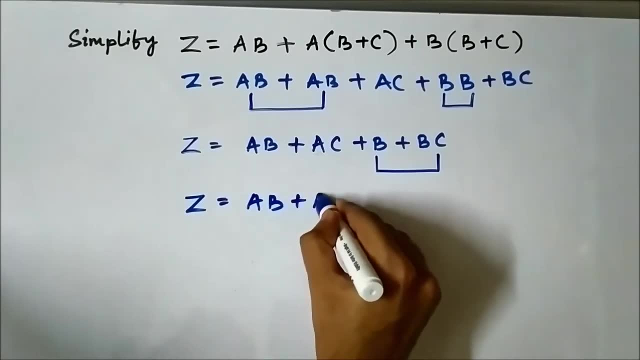 the basic concepts related to Boolean algebra. so again we can write it as a, b plus a, c plus b. okay, now again these two terms, a, b and b. again we can apply the same thing: b plus b, a, or b plus b, a b, whatever it will result. 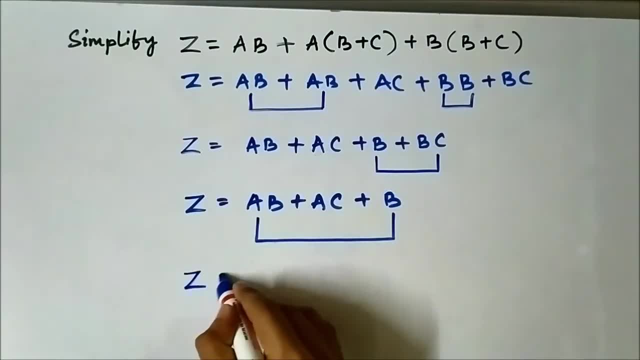 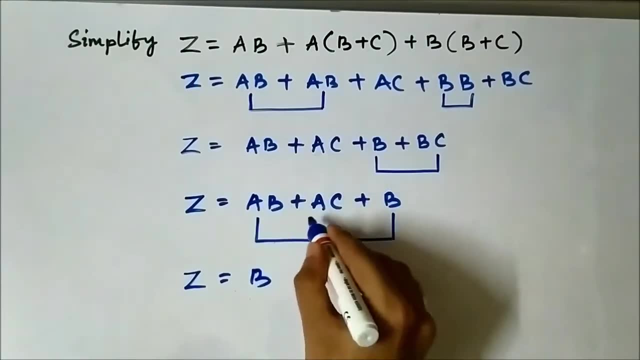 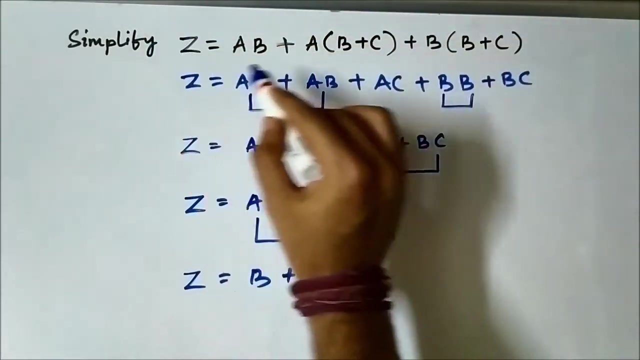 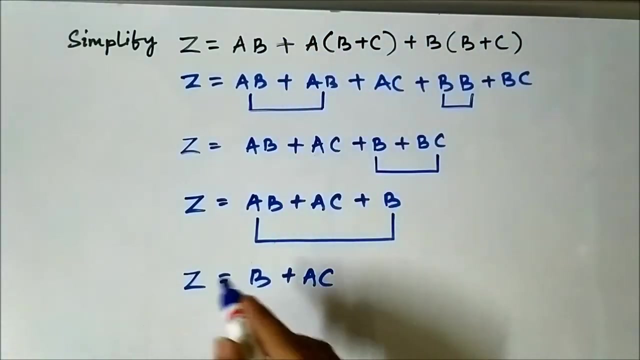 in b using the same rule. so here it will be b, this two, a, b plus b. it will be b plus a c. this is the final simplified expression. so we have reduced this Boolean expression, which consisted of many Boolean variables and terms, into this. okay, this is the simplified or reduced version of this Boolean expression. 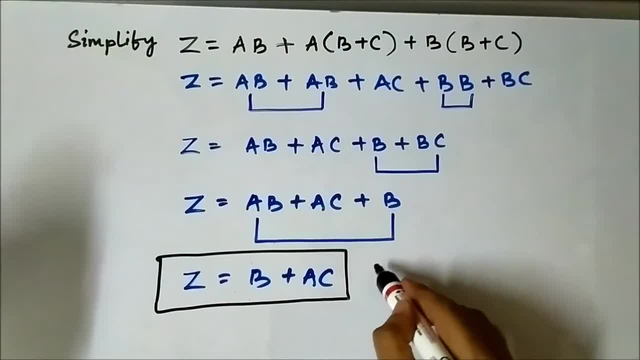 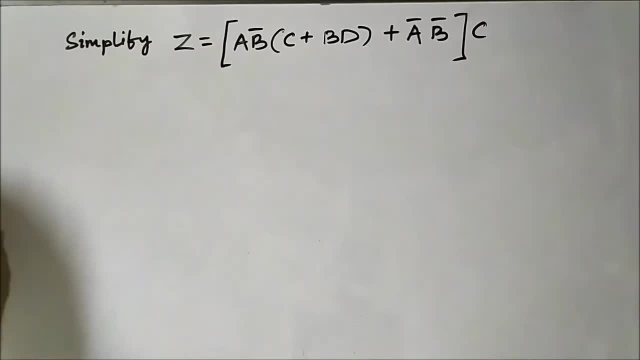 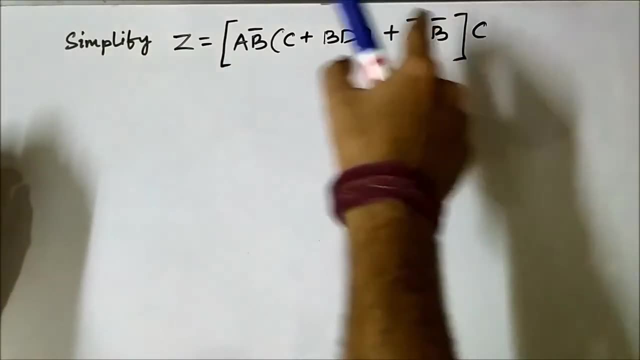 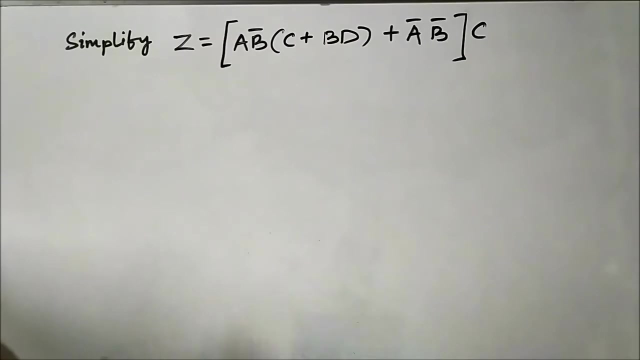 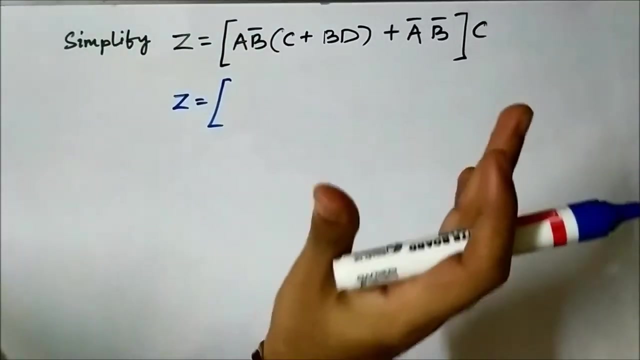 b plus a c. this is our final expression. okay, so here we will solve another Boolean expression. we will simplify it. so here is this Boolean expression. now we have to simplify it using the rules of Boolean algebra. okay, so let us keep this square bracket in tact and let us open the inner brackets, okay. 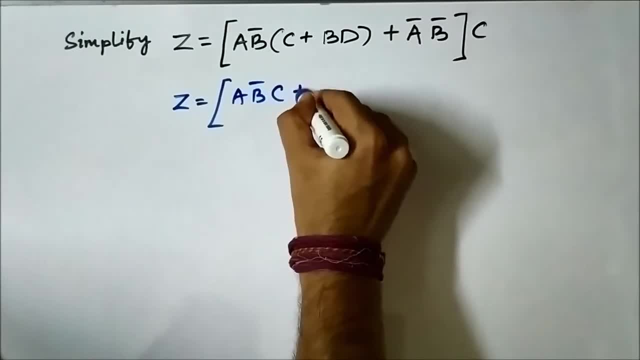 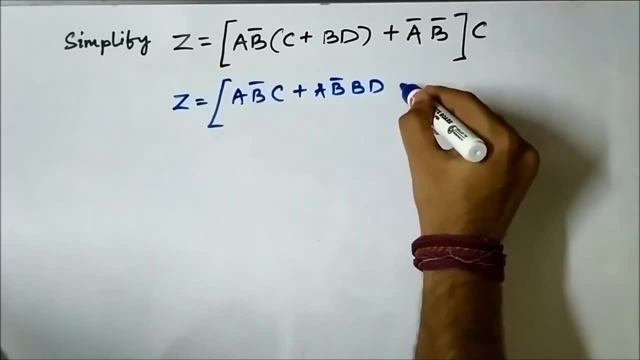 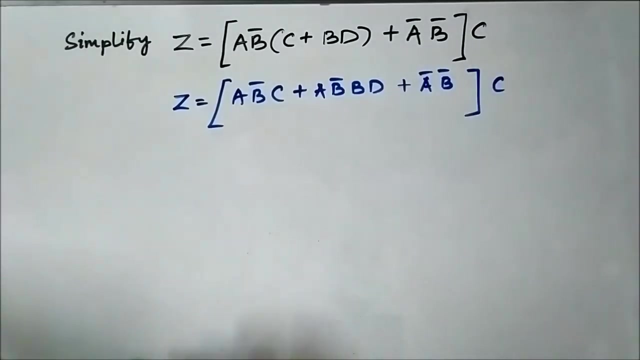 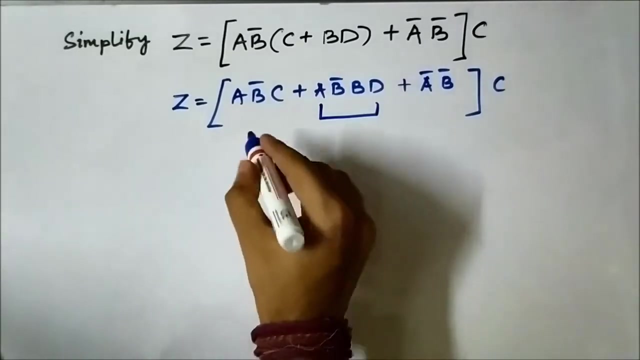 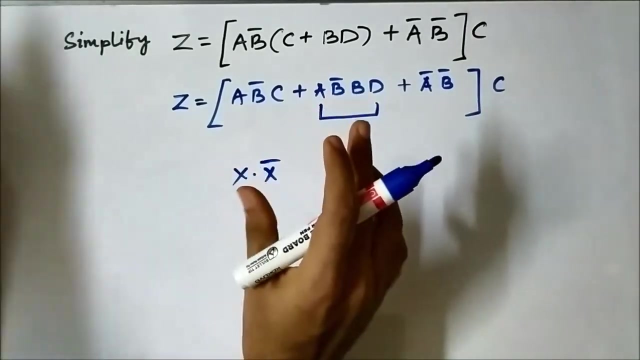 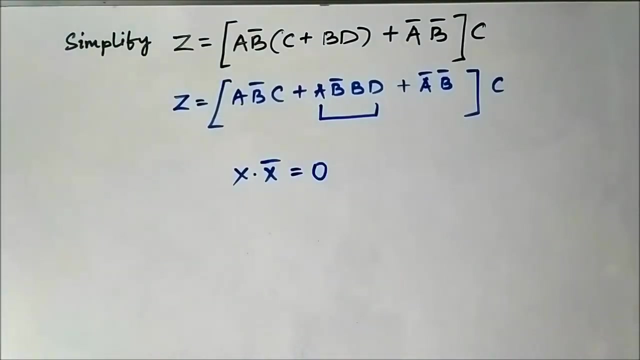 a b bar c plus ab bar p, d, a bar b bar c. Now focus here. we have one AND rule which says if a Boolean variable is multiplied or ANDed with its complemented variable, it will result in 0. So we will apply this rule here. 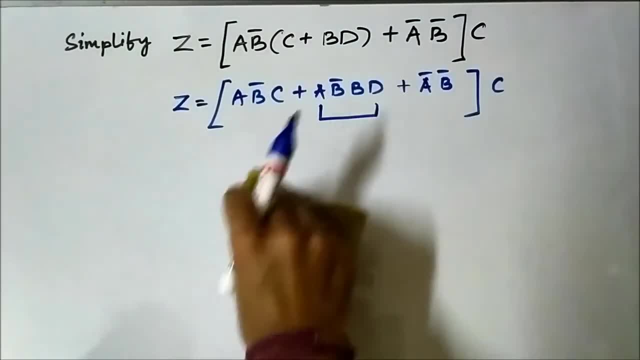 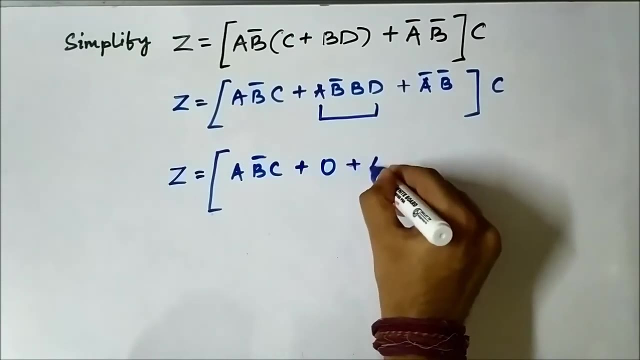 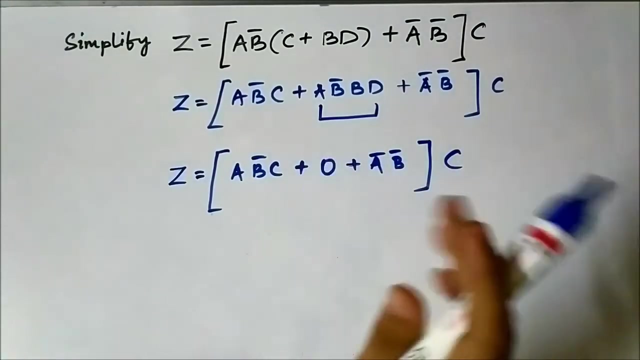 So this term will become 0.. So we can write it as: z is equal to a b bar c plus 0, plus a bar b bar c. So plus here again. I will repeat: plus here means or into, or multiplication, or product here. 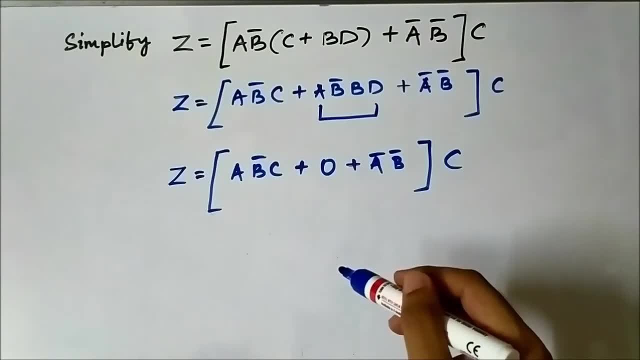 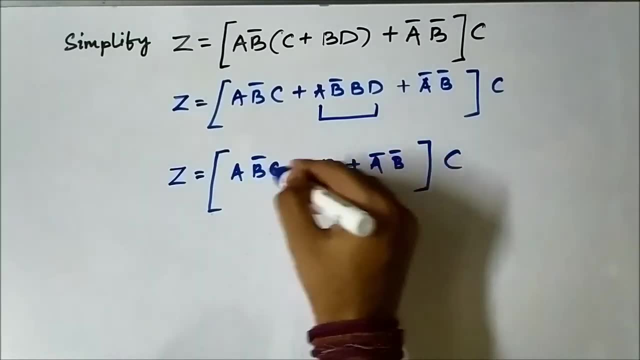 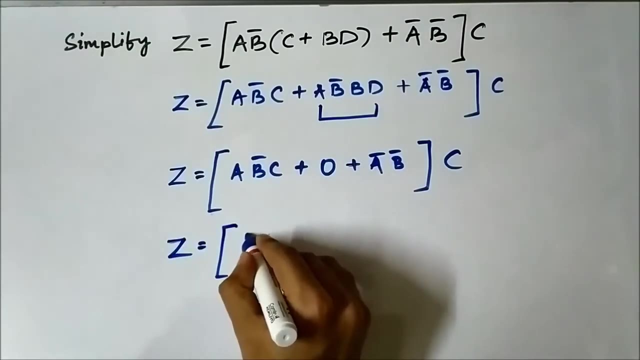 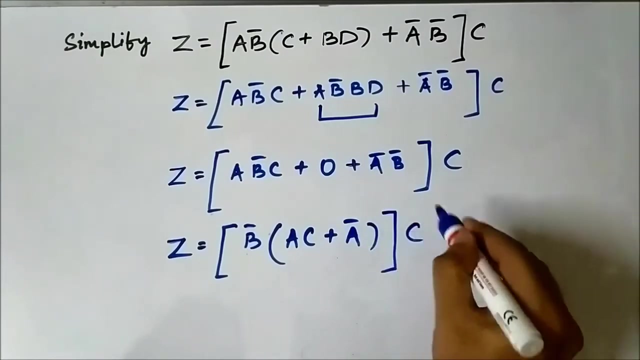 is. AND Now here these two terms, here b bar, is common in both of them, So we can write it as b bar into a, c plus a bar Into c. Now we have a rule which is something like this: which is: x plus x bar, y is equal to x plus y. or we can write it in this way: x bar. 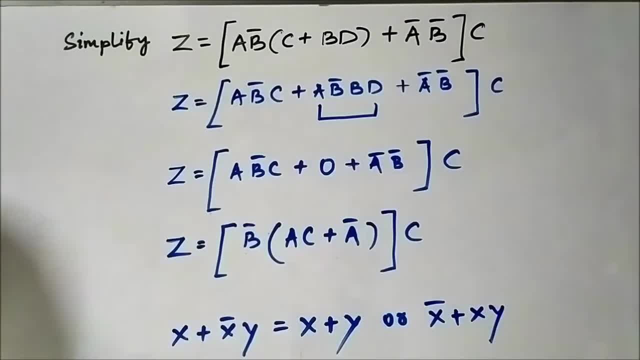 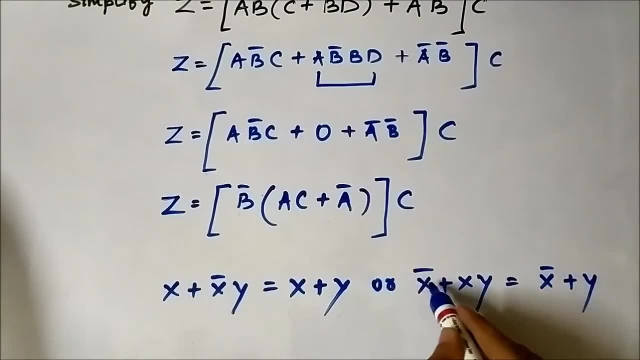 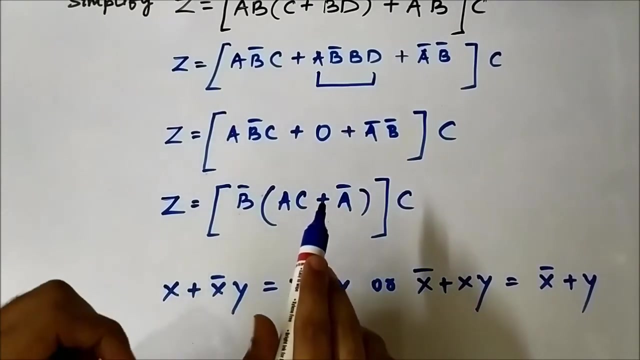 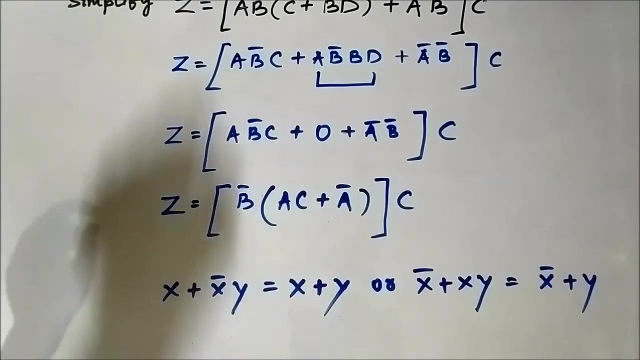 plus x y is equal to x bar plus y. So this rule is applicable here: a bar plus a c, a bar plus a c. So here it will be a bar plus c, it will be a bar plus c. so let us do that. 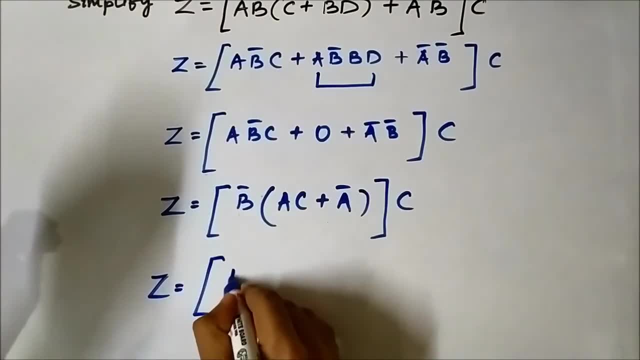 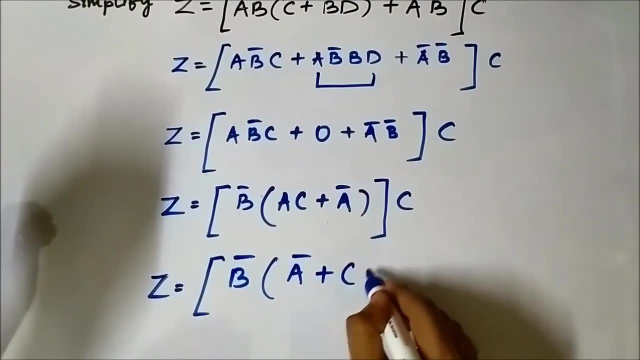 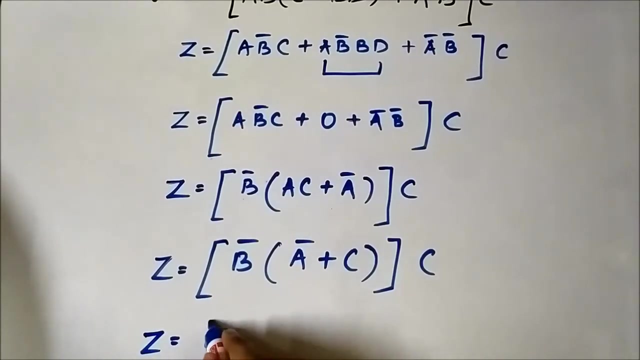 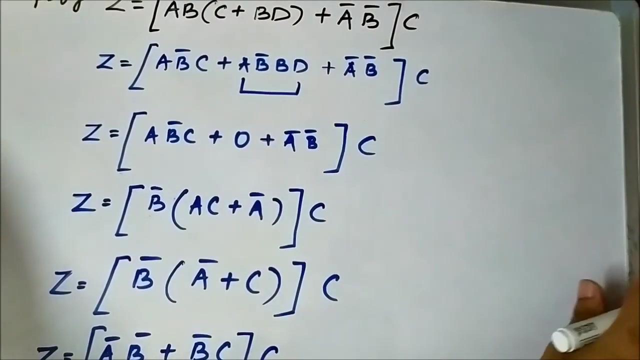 So it will be equal to b bar into a bar plus c into c. So here it will be: z is equal to a bar b bar plus b bar c into c. So now it will be, if we can write it here: z is equal to. 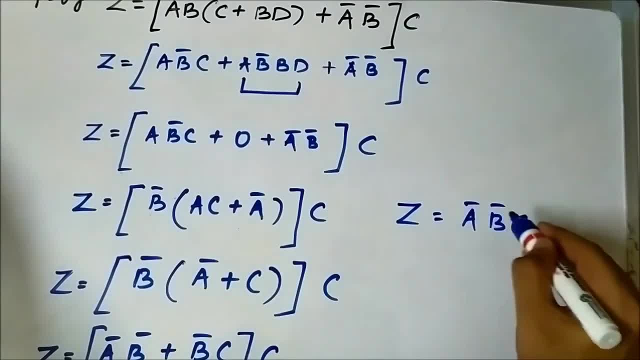 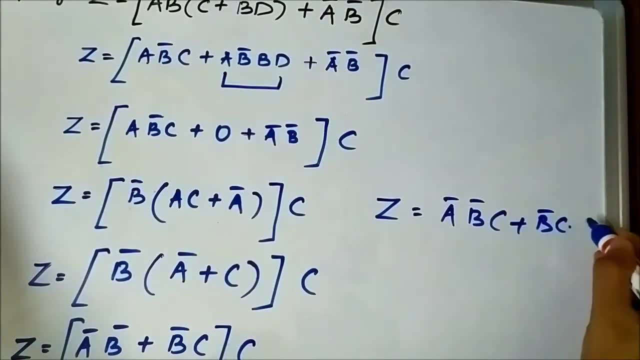 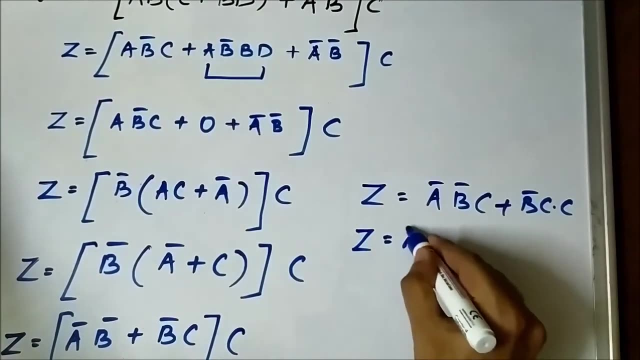 a bar b bar c. We are opening the bracket plus b bar c, c, c into c, it will result in c, So it will be. z is equal to a bar b bar c plus b bar c. Now here b bar c is common, So it will be.